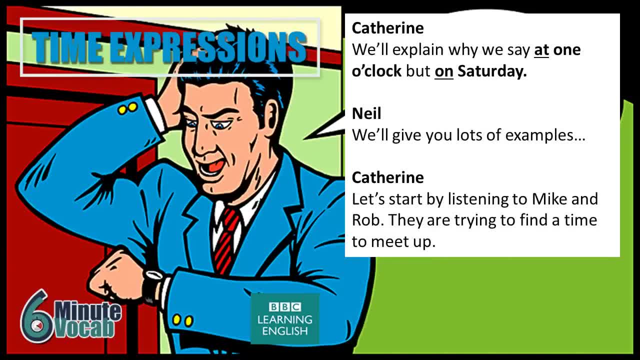 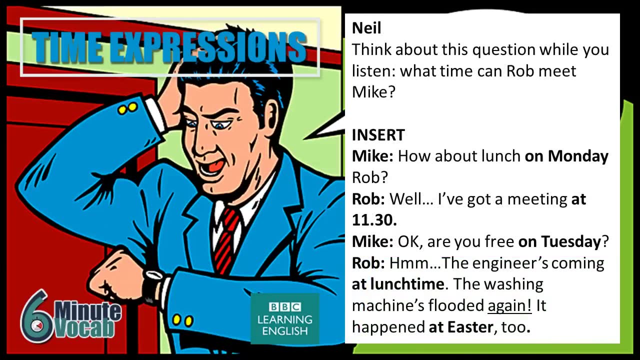 We'll explain why we say at one o'clock, but on Saturday Yes, and we'll give you lots of examples. Let's start by listening to Mike and Rob. They're trying to find a time to meet up. Think about this question while you listen: What time can Rob meet Mike? 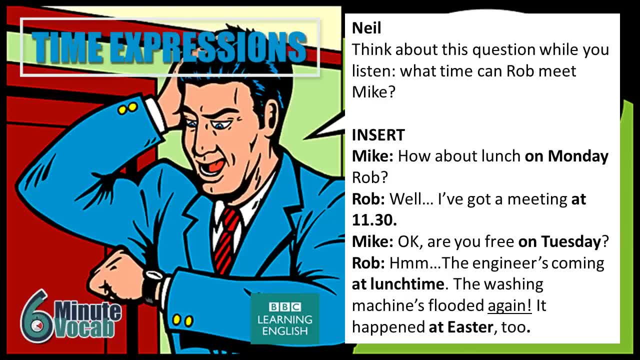 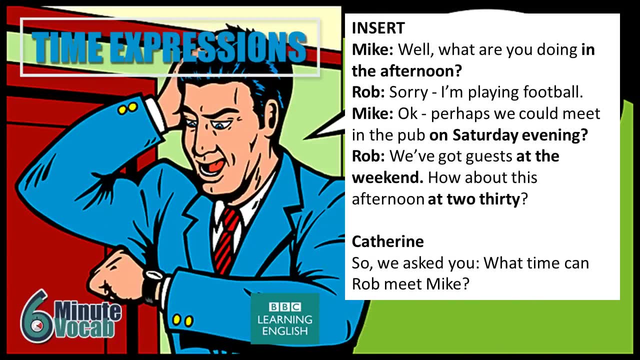 How about lunch on Monday, Rob? Well, I've got a meeting at 11.30.. OK, Are you free on Tuesday? The engineer's coming at lunchtime. The washing machine's flooded again. It happened at Easter too. Well, what are you doing in the afternoon? 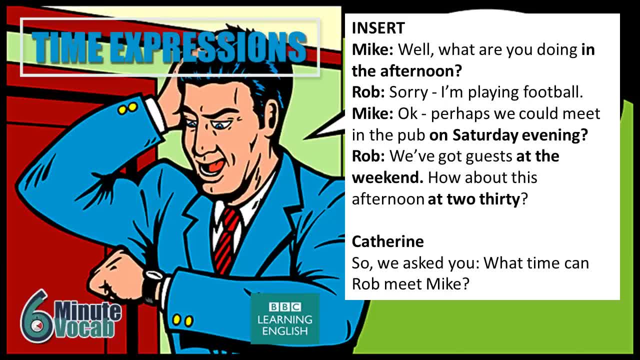 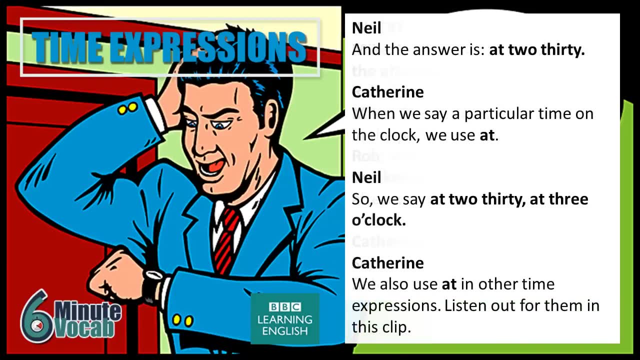 Sorry, I'm playing football. OK, Perhaps we could meet in the pub on Saturday evening. We've got guests at the weekend. How about this afternoon at 2.30?? So we asked you what time can Rob meet Mike? And the answer is at 2.30.. 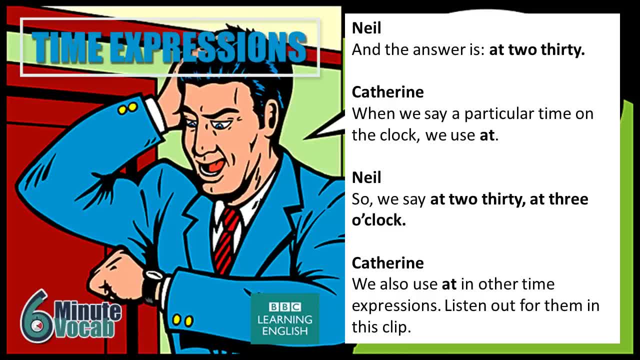 When we say a particular time on the clock we use at, So we say at 2.30, at three o'clock. We also use at In other time expressions. Listen out for them in this clip. How about lunch on Monday, Rob? 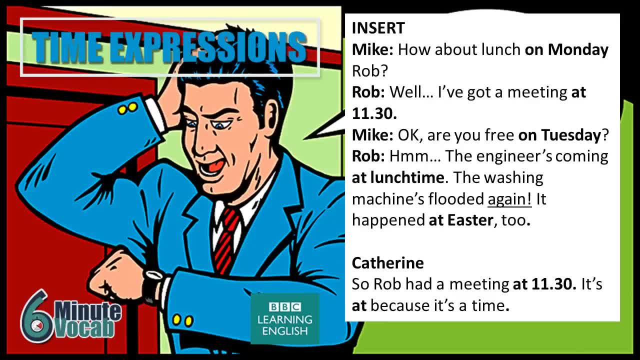 Well, I've got a meeting at 11.30.. OK, Are you free? on Tuesday, The engineer's coming at lunchtime. The washing machine's flooded again. It happened at Easter too. So Rob had a meeting at 11.30.. It's at because it's a time. 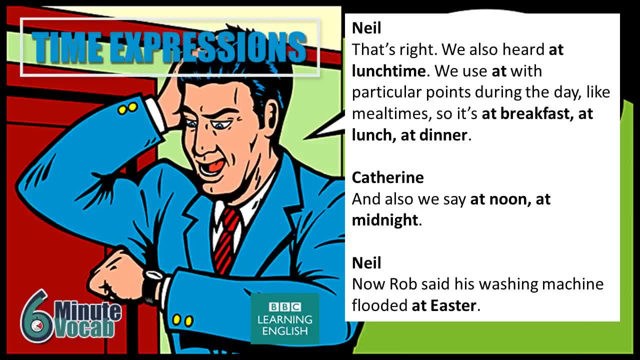 That's right. We also heard at lunchtime. We use at with particular points during the day like mealtimes, So it's at breakfast, at lunch, at dinner, And also we say at noon, at midnight Now Rob said his washing machine flooded at Easter. 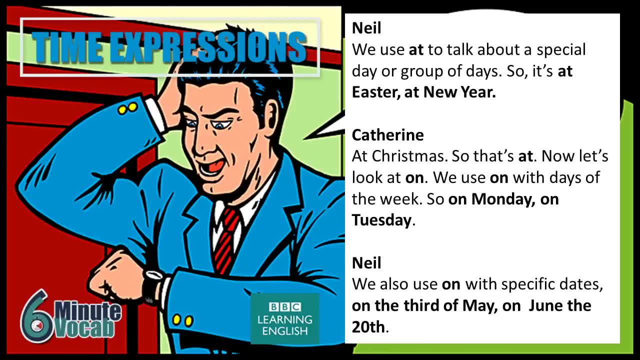 We use at to talk about a special day or group of days. So it's at Easter, at New Year, At Christmas. So that's at Now, let's look at on. At Christmas: So that's at Now, let's look at on. 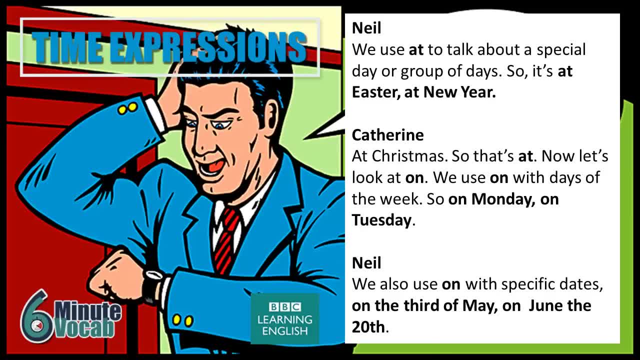 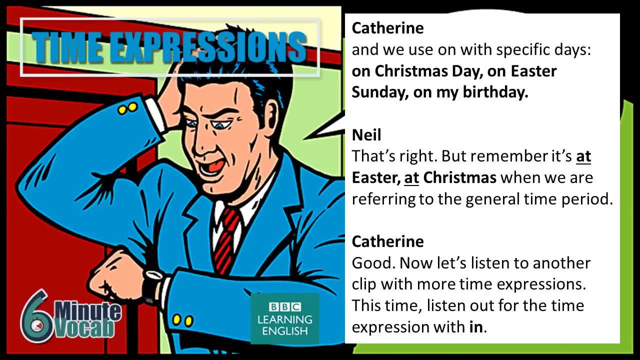 We use on with days of the week, So on Monday, on Tuesday We also use on with specific dates On the 3rd of May, on June, the 20th, And we use on with specific days On Christmas Day, on Easter Sunday, on my birthday. 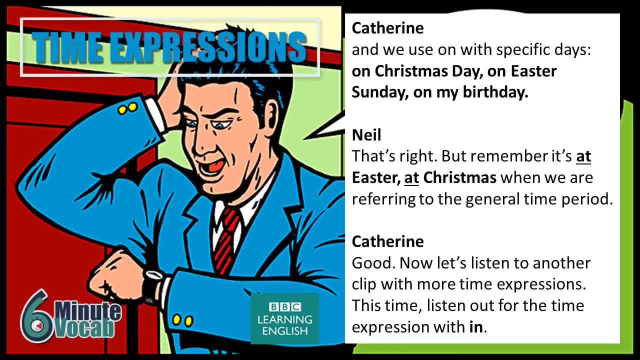 That's right, But remember it's at Easter, at Christmas, when we are referring to the general time period. Good, Now let's listen to another clip with more time expressions. This time listen out for the time expression with in. 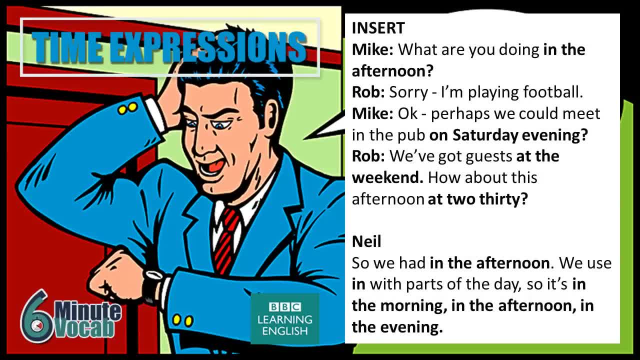 What are you doing in the afternoon? Sorry, I'm playing football. Ok, Perhaps we could meet in the pub on Saturday evening. We've got guests at the weekend. How about this afternoon at 2.30?? So we had in the afternoon. 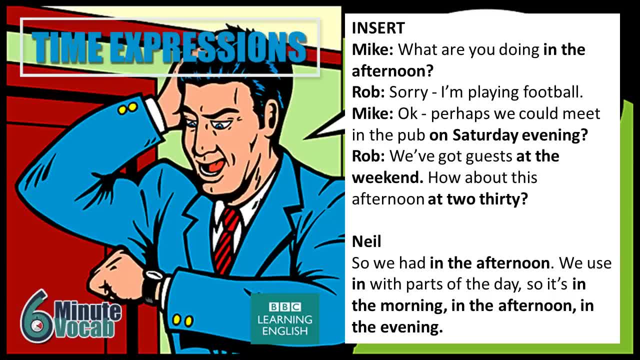 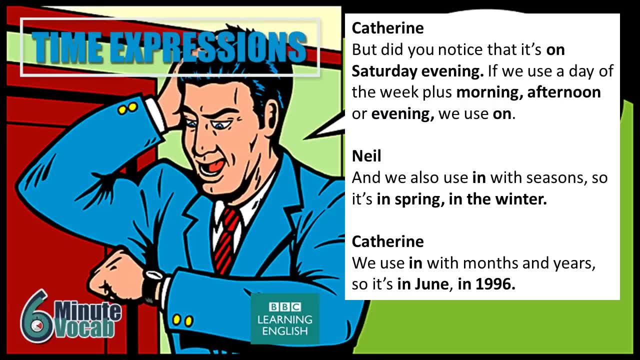 We use in with parts of the day. It's in the morning, in the afternoon, in the evening. But did you notice that it's on Saturday evening? If we use a day of the week plus morning, afternoon or evening, we use on. 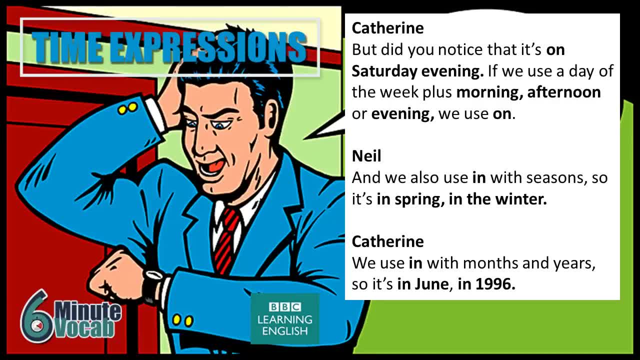 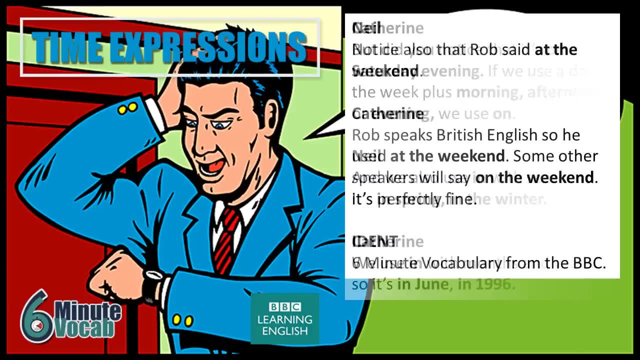 And we also use in with seasons, so it's in spring in the winter. We use in with months and years, so it's in June in 1996.. Notice also that Rob said at the weekend. Rob speaks British English, so he used at the weekend. 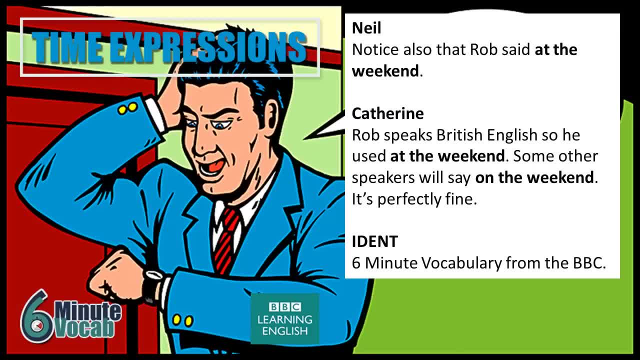 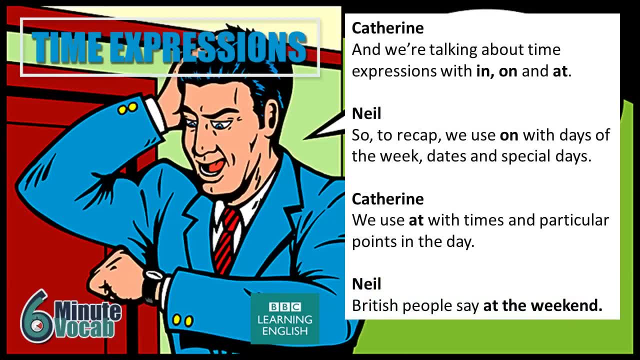 Some other speakers will say: on the weekend It's perfectly fine. Six Minute Vocabulary from the BBC And we're talking about time expressions with in, on and at We are. So, to recap, we use on with days of the week. 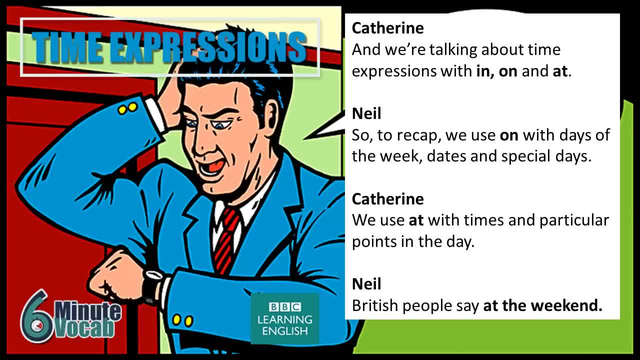 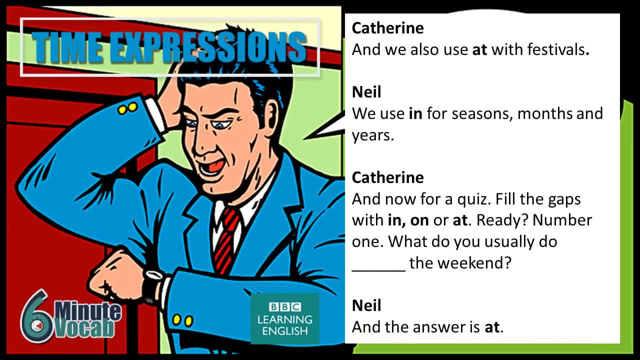 Dates and special days. We use at with times and particular points in the day- British people say at the weekend- And we also use at with festivals. We use in for seasons, months and years. And now for a quiz: Fill the gaps with in on or at Ready. 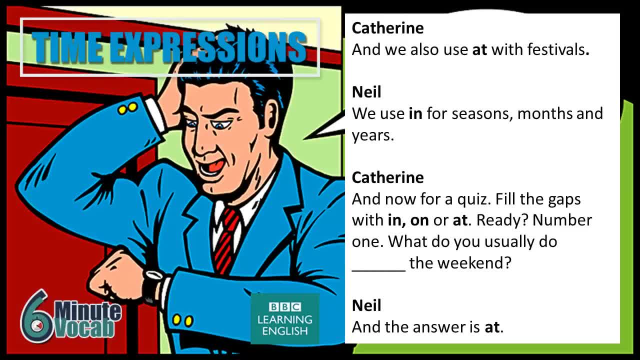 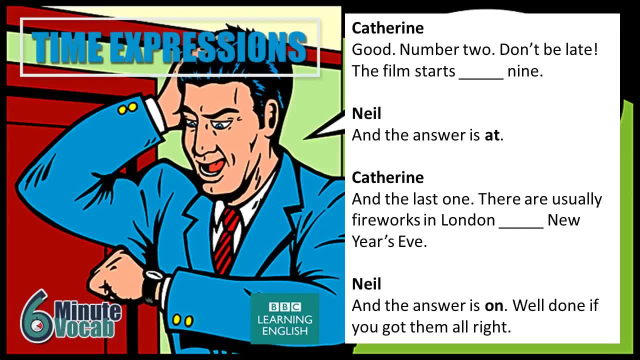 Number one: What do you usually do the weekend? And the answer. And the answer is at. Good Number two: Don't be late, The film starts nine And the answer is at. And the last one: There are usually fireworks in London New Year's Eve.